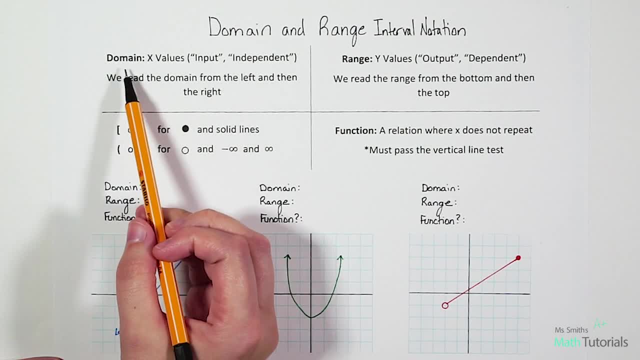 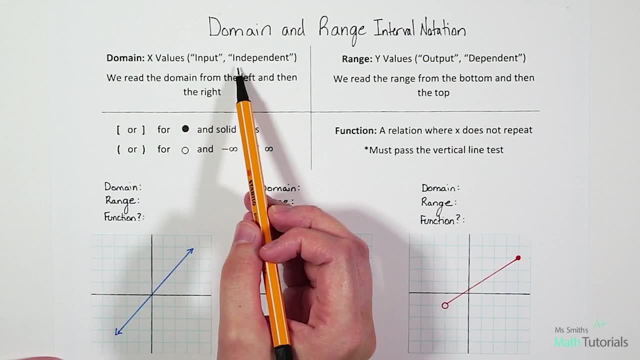 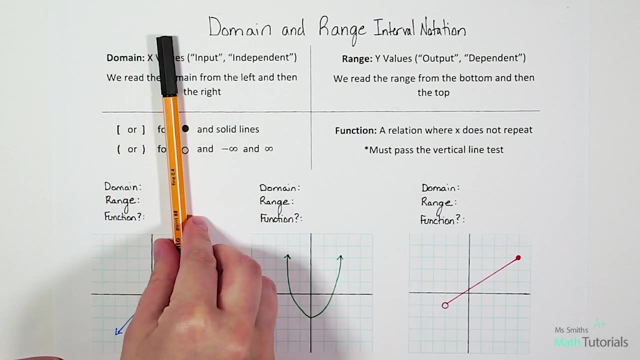 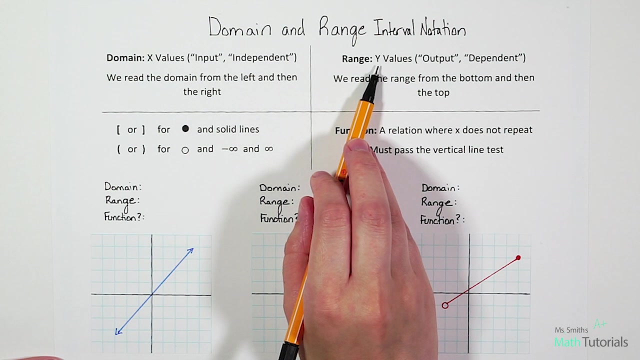 is what is domain and what is range. Domain is just another way of saying the x values. Other common words are input and the independent. We will always read domain on a graph from left and then right For our range. that's all of our y values, So we're focusing on the y-axis. 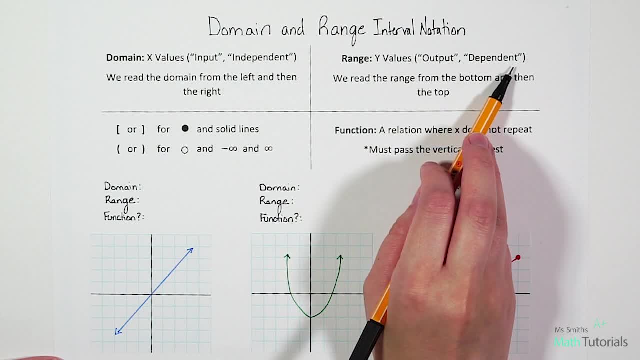 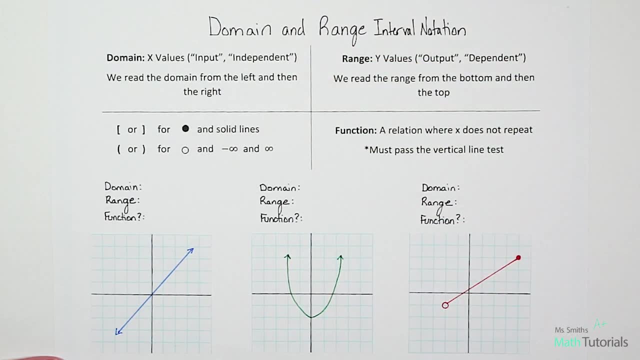 It's also known as the output or the dependent. We read the range from bottom and then top, So really all your questions are about the range, So we're going to be focusing on the y-axis. you need to know to be able to answer domain and range for interval notation. is that we're going? 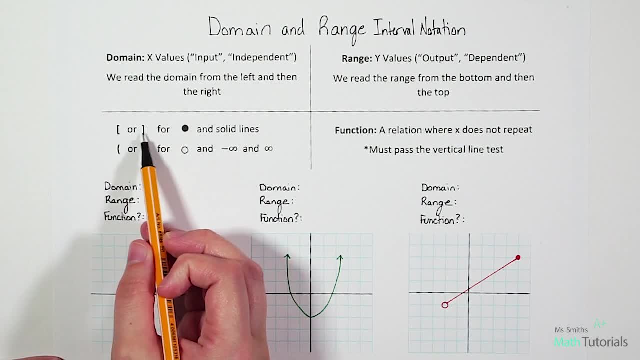 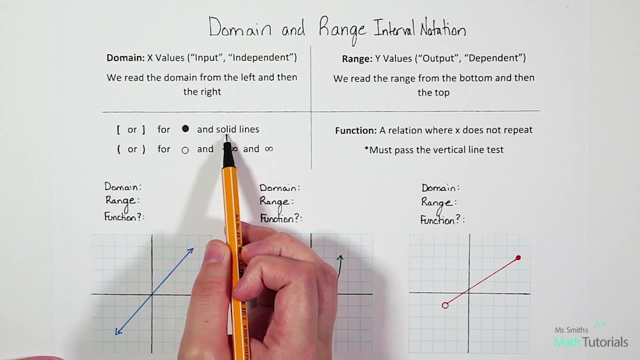 to use brackets, So it could be a bracket facing this way or this way, depending on the situation. We use brackets for solid points and solid lines, So if you ever see a solid line that's made up of solid points, So it always won't be like a point on the graph, but a solid line counts as. 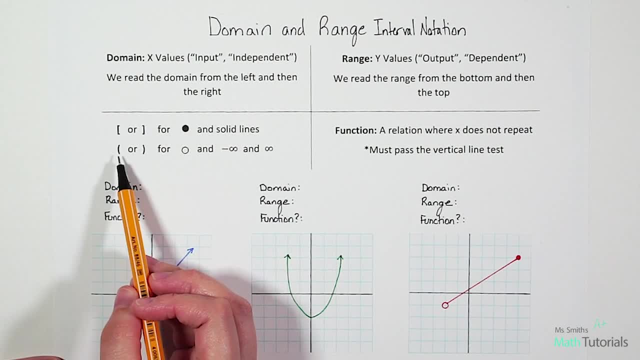 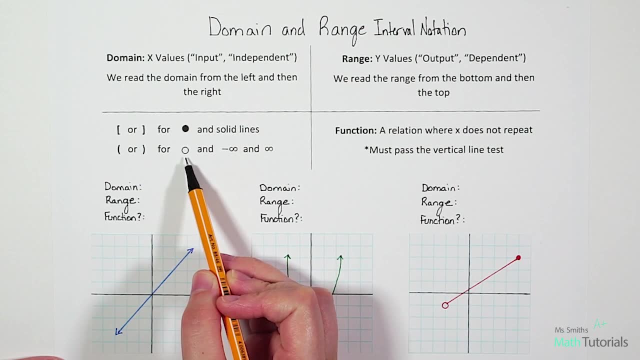 a solid point, We'll also use parentheses, and we use parentheses for if we have an open point, We also use parentheses if we use a negative infinity or a positive infinity. The reason we would use parentheses and not brackets is because the open circle shows a 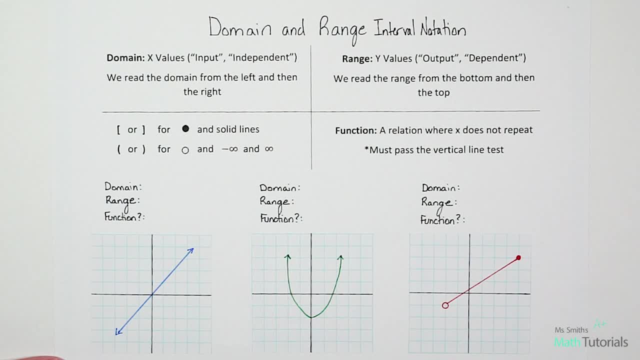 non-included point. Infinity is more of an expression. It just means that it keeps going on for infinity. Infinity is not a place or a point that we reach, which is why we always use parentheses like our non-included points, for infinities. 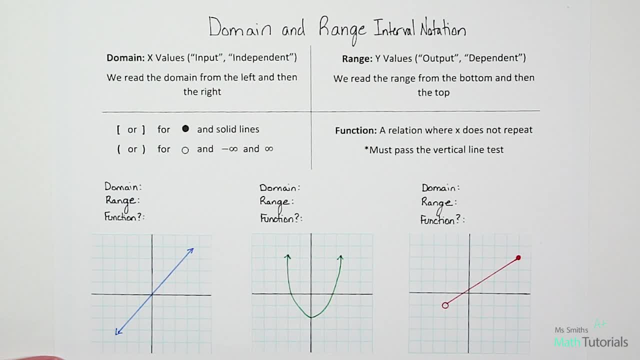 The last thing we'll need to know to be able to answer each of these questions is: what is a function? So, a function is a relation where x does not repeat Each of our graphs. in order to be a function, they have to pass. 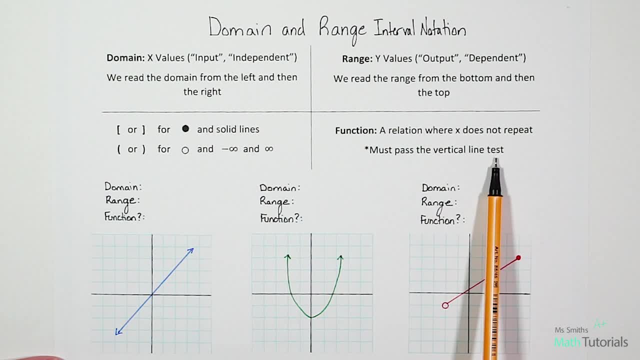 The vertical line test. So we use a vertical line test to see: does the graph cross our pin more than once? when we hold our pin in a vertical line, I think it's a little easier to understand once we actually see it in a problem. So let's dive right into some examples. 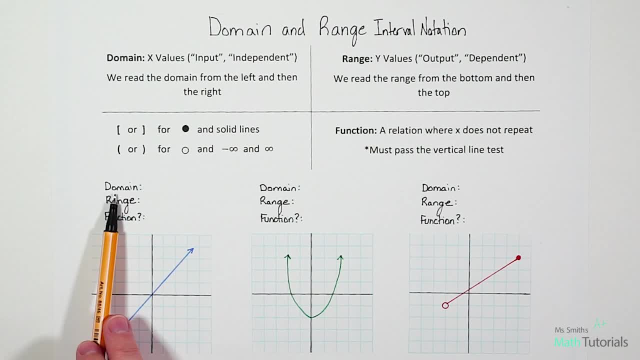 When we look at this first example, the first thing that they're going to ask us for is the domain. Now, remember, we said domain is our x values. So when we look at domain, we're looking at the x-axis values. We do not care about the y-axis at all when we're doing domain. Remember. 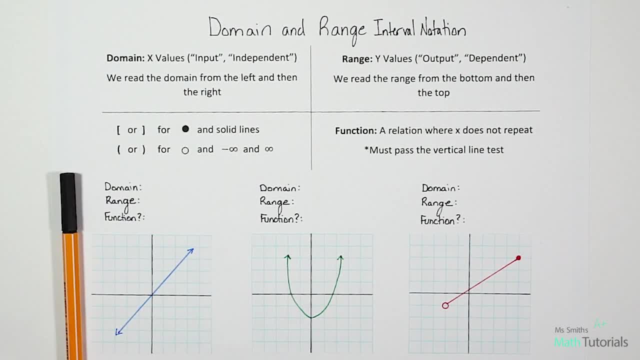 that we also said we read domain from left to right. okay, So when we read it from the left, we're going to just take our pin and pull in and we ask ourselves what's the first place that we hit. Now some students would say, oh, we're hitting at. 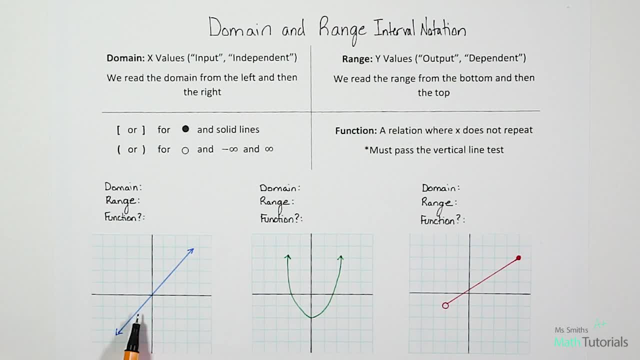 negative three. But here's the thing. That's where our blue arrow looks like. it's, you know, at a stopping point. But here's the thing. It's an arrow And arrows keep going on forever. It doesn't stop there at negative three. It's going to keep going on and on to infinity. 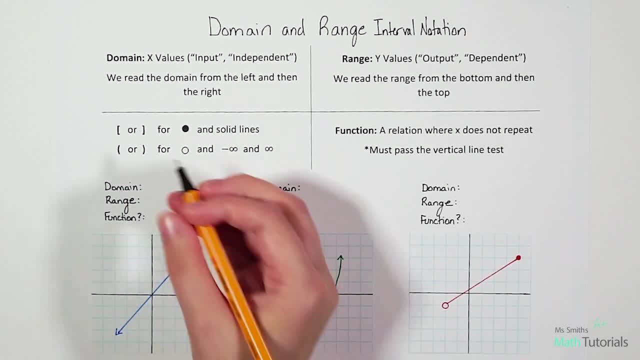 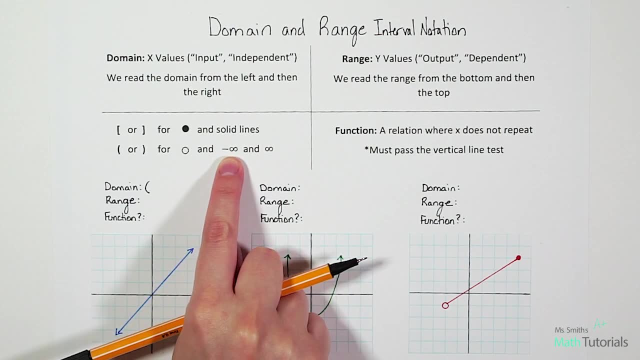 So we're going to use a parenthesis And because it's on the left, it's going to be negative infinity For our x-axis. this direction is negative infinity. This direction is positive infinity. We read from the left. Now let's read from the right. What's the first place I touch? 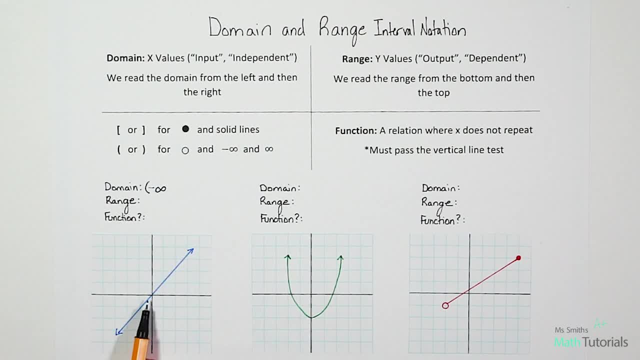 Another arrow. This time it's pointing in this direction. So it's going to be positive infinity, And how we show this is we put a comma and then we put positive infinity And you don't need to do a plus for positive. Sometimes people do, and that's fine, But by just 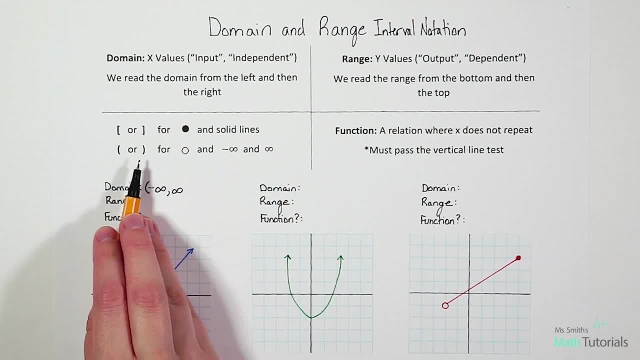 putting infinity, it's understood that it's positive And remember, infinities always get parentheses. So that is our domain for this graph. It reads: from negative infinity to positive infinity. Another way to say negative infinity to positive infinity is using this: 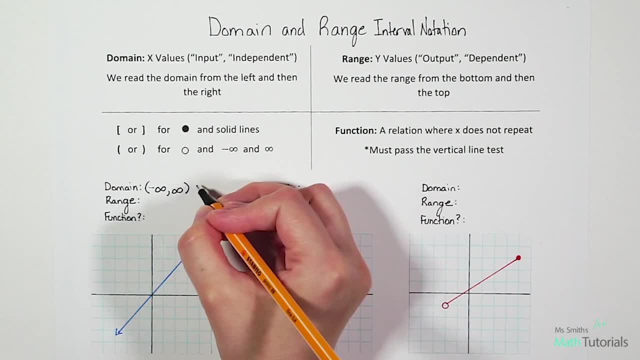 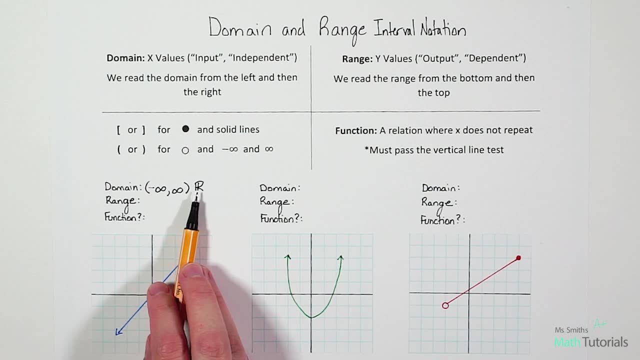 symbol right here. I always think of it as a double-lined R. We do two lines and then we put an R, And what that stands for is all real numbers. That's another way to say the same thing. It's just a little less writing and a little shorter. So you may see that symbol. You could also write. 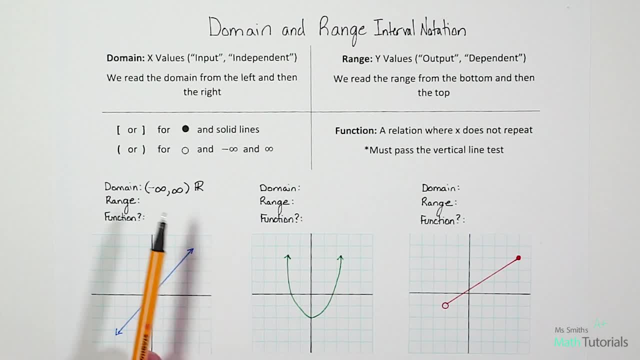 out all real numbers if you wanted to. That's fine too, But either one of these answers is acceptable if it is a negative infinity. So if it's a negative infinity, then it's a positive infinity. To a positive infinity, it has to be both Okay. so let's look at the range now. So remember: 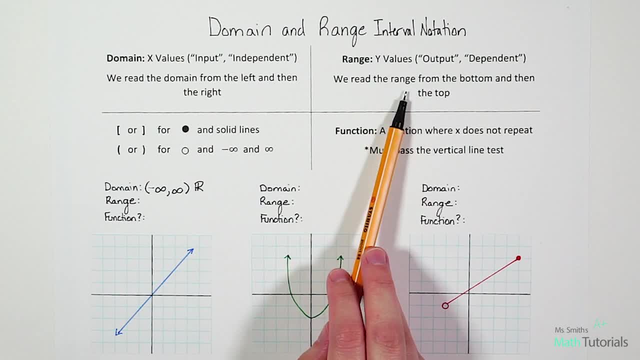 ranges are y values and we read the range from bottom and then the top. So now we're looking at our y-axis. We don't care about x anymore, just y. So we always read from the bottom and we pull up. What's the first place we hit? We hit an arrow. Arrow means infinity. Now, because the 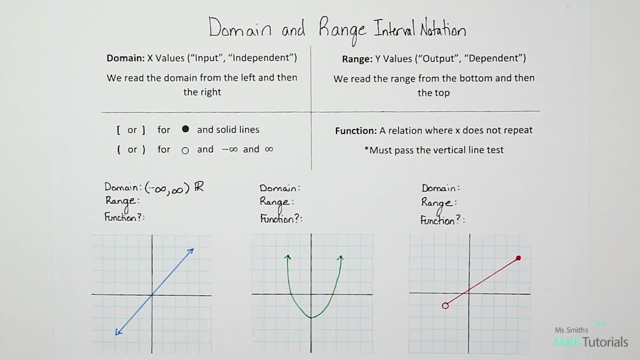 y-axis is on the left side. we're on the left side, right, This is going down. We call it negative infinity. Okay, now we read from the top And what's the first place? we hit Another arrow. An arrow means infinity. It's on the right side of our answer and it's pointing up, So it's called. 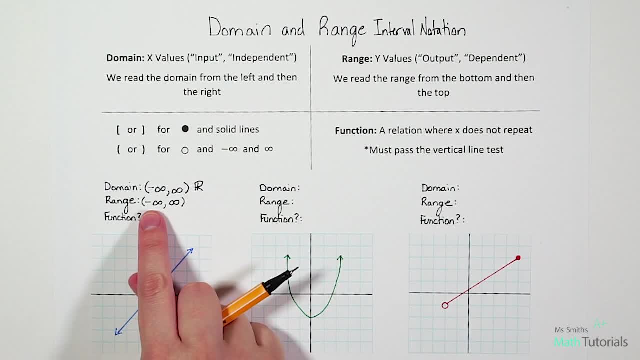 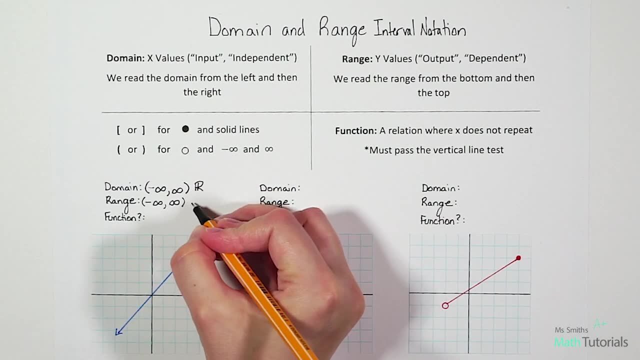 positive infinity. Now notice again: we've got negative infinity and we've got negative infinity. So we're on the right side of our answer and it's pointing up. So it's called positive infinity. So if we wanted to, if we recognized that early, we could also just put our answer as: 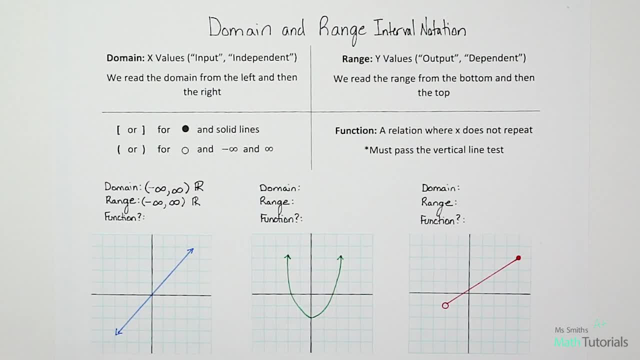 all real numbers. A good thing to note here is, if it confused you at all with: oh, I'm not sure if I should use negative infinity or positive infinity. If it's on the left, it's always going to be negative infinity, And if it's on the right, it's always going to be positive infinity. 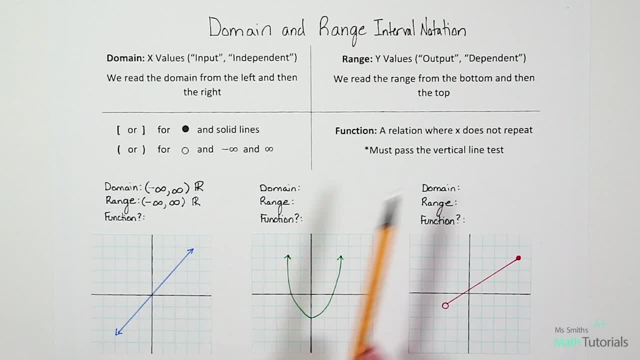 Okay, now we ask ourselves: is this a function? So now we're going to go into that- must pass the vertical line test. What the vertical line test is is use. a great object to use is your pen, because your pen can form a perfect vertical line. And we take the. 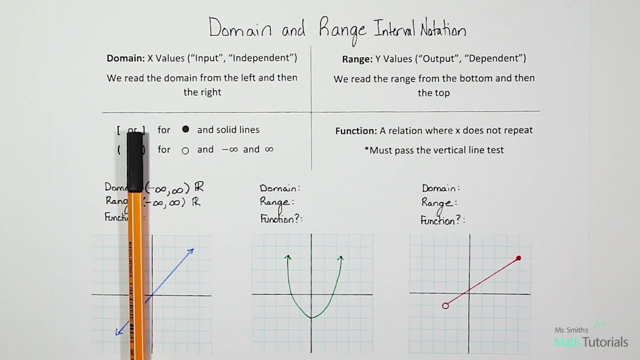 vertical line and we run it through the graph And what we're testing is: does the blue line hit my pen more than once at a time? And if we run it through we see no, it's only ever hitting my pen once at a. 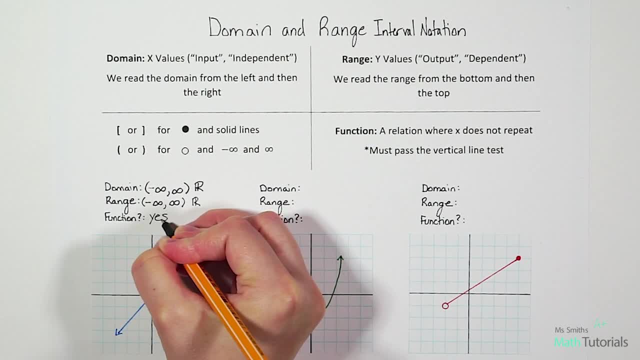 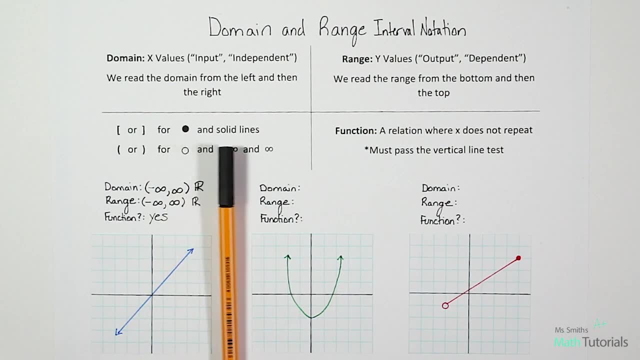 time. So, yes, This is a function, Let's do another one. So for domain, for this one, remember, we read domain left and then right. So when I read from the left, what's the first place I hit? I hit an arrow. 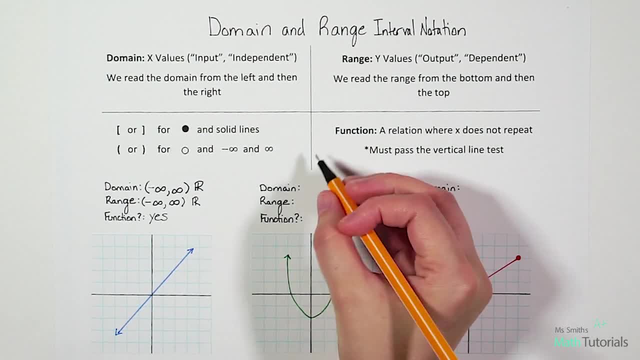 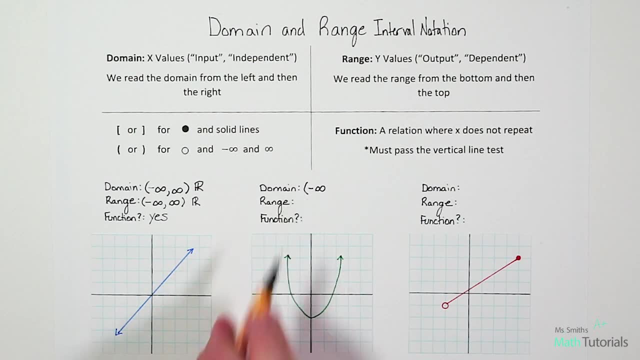 and an arrow means infinity. Now it's on the left, So we know it's going to be negative infinity, And remember infinities always get parentheses. See what happens on the right, So we're going to come in from the right. what's the first place we 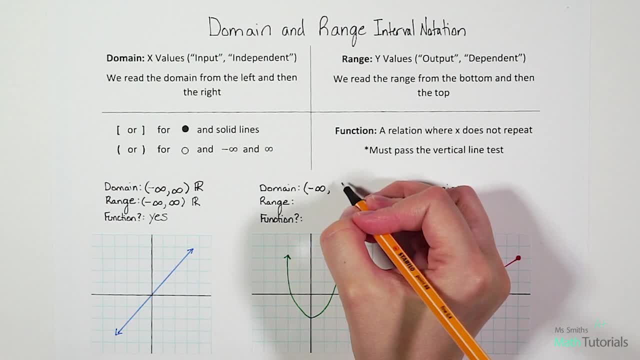 hit Another arrow. So we know arrow means infinity. And because it's on the right, we know it's going to be positive infinity and it gets a parentheses. And because we got that double infinity, we could say all real numbers if we wanted to. For our range, remember range we start. 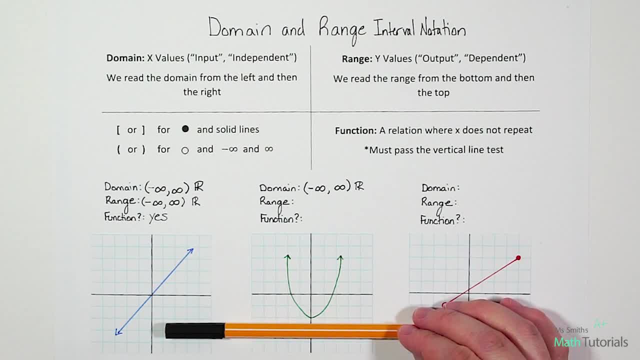 from the bottom And what's the first place we hit? Okay, this is the first time we haven't hit an arrow. So what did we hit? Well, if we're looking at our y axis, remember we don't care about x at all, we're doing the range. So when we look at the 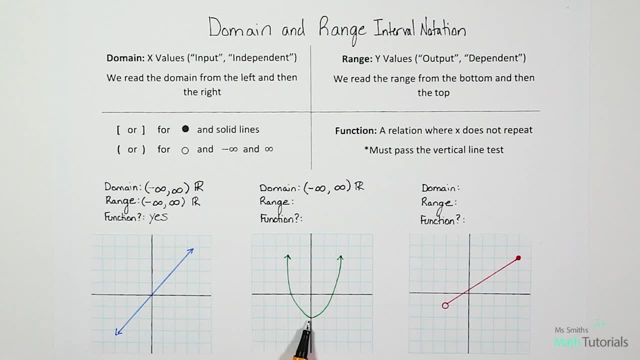 y axis. what is that? first place we hit Negative two. So then we ask ourselves: okay, is it a solid point at negative two Or is it an open point? Now I will say, if it's an open point it will very. 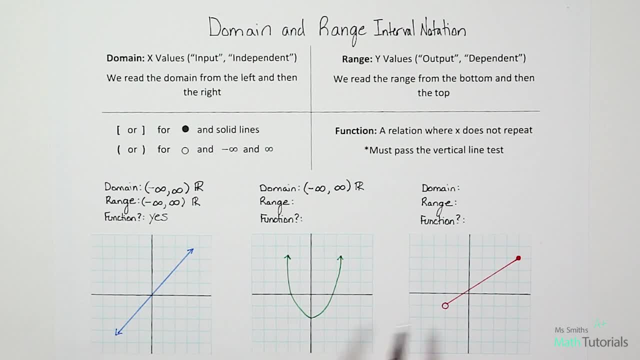 obviously be an open point, Kind of like this: This is just a solid line, So remember, solid lines get brackets. So our piece with the negative two, we'll get a bracket. Now let's see what happens when we come from the top. What's the first place we hit? Now, in this case, we hit two arrows. 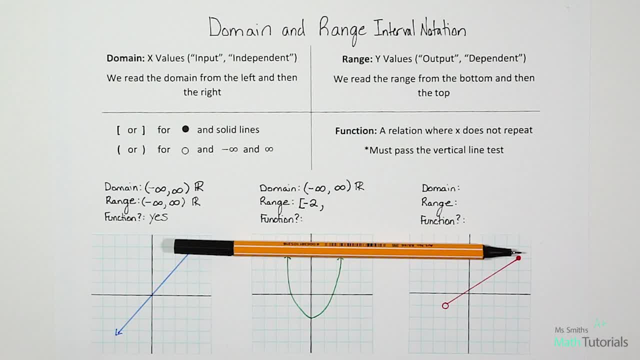 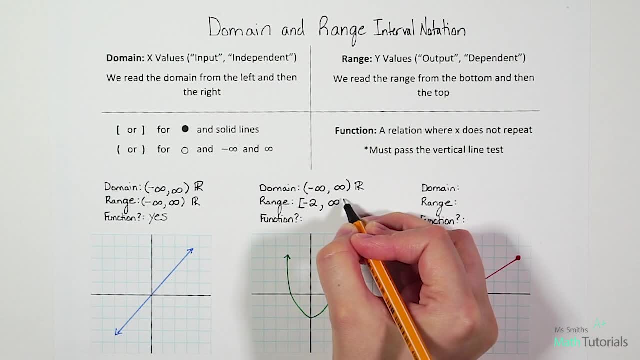 that doesn't matter. as long as you hit one arrow, two arrows, it doesn't matter. an arrow going up means positive infinity, which always gets a parenthesis. So we could not do an all real numbers symbol here, because we don't have double infinity. 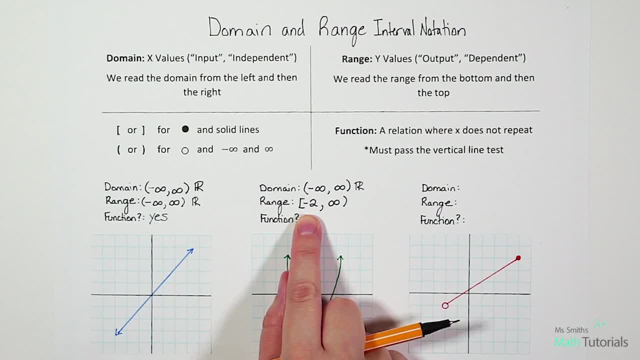 We've got positive infinity, but over here we didn't. We could not say all real numbers. Now is this a function? Does it pass the vertical line test when we pass our pin through it? It's only ever hitting my pin once at a time. 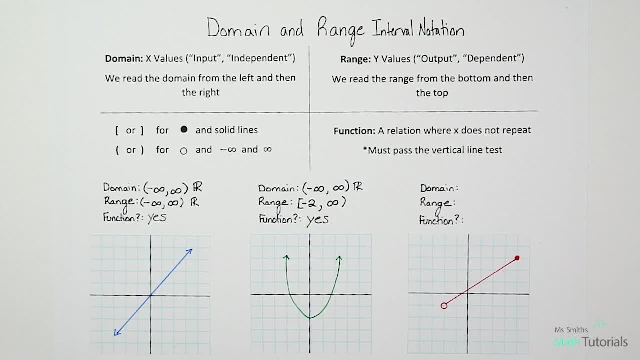 So, yes, this is a function. Okay, for this next example, when we ask for our domain and we look from the left, the first place we hit is an open circle. And where is that open circle? Remember, domain means x, so we're looking at the x. 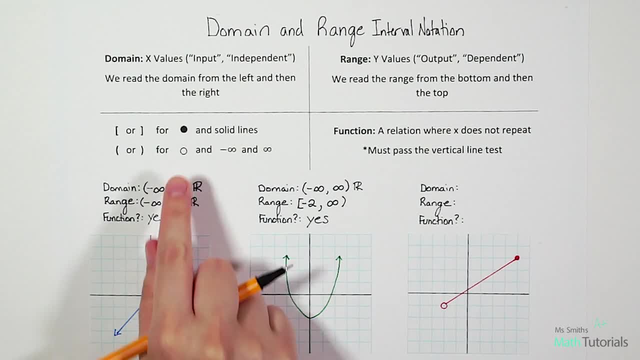 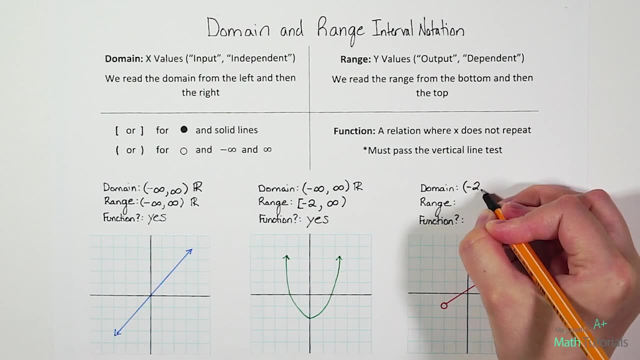 It falls at negative two. So remember: open circles get parentheses. So we're gonna do a parentheses, negative two and negative one. Let's see where we end up on the right. So when I pull in from the right, what's the first place I hit? 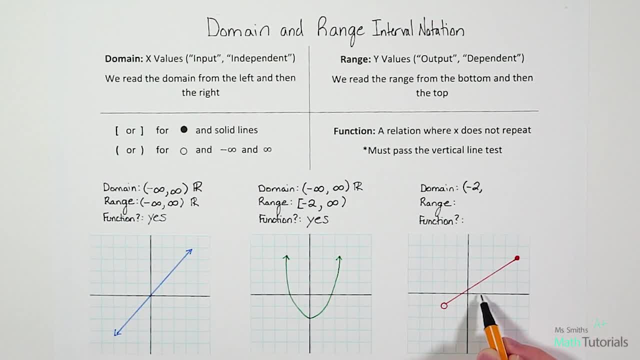 It's a solid point. at positive one, two, three, four- Remember solid points get brackets For our range. let's look from the bottom up. What's the first place we hit? It's an open circle. at negative one, 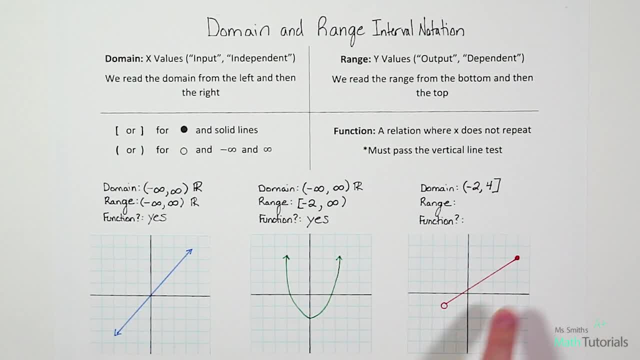 Remember, for range we care about the y-axis, Not the x. So we hit negative one And open circles always get parentheses. And then when we measure from the top, what's the first thing we hit? It falls at one, two, three positive three. 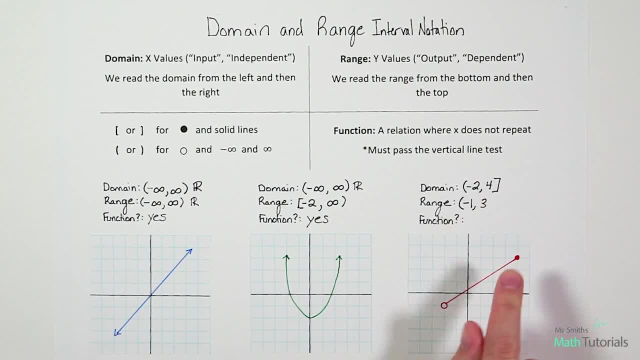 We look at the y-axis And it is a solid point at positive three. so it gets a bracket. Now is this a function? Does it pass the vertical line test? Yes, that red line is only touching our vertical line once at a time. 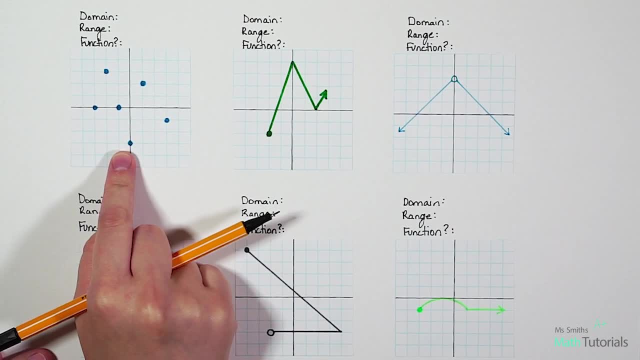 Let's look at some more examples. This one looks very different from all the other graphs and from the ones we did on the first page. This one just has random points, Now what we should not do, but what I see a lot. 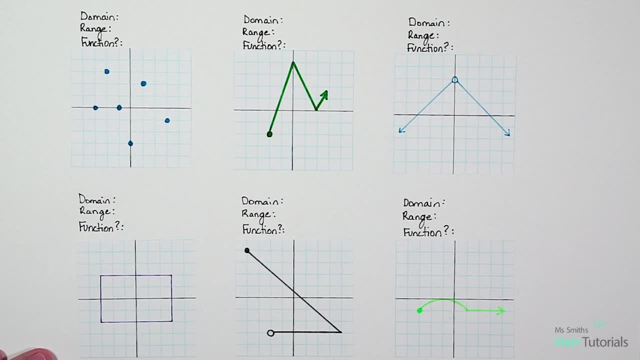 is people wanna just connect the dots and then they're like, oh, that's not good, So we're gonna make them connect the dots and make their own line. We don't wanna do that right. We are just given points, not any type of line. 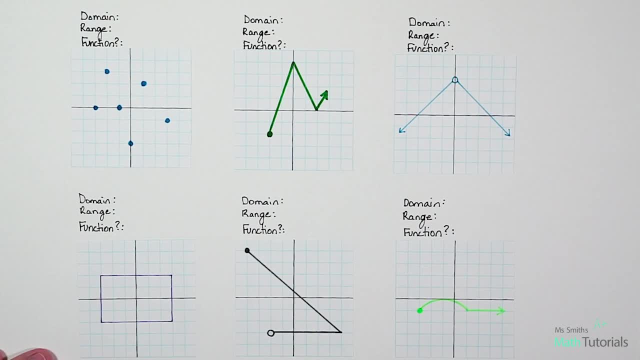 So we do not connect them. But these ones are actually the easy ones, I think, For domain. they're just asking for all the x values, So all we need to do is list in a set. And here's how we do a set. 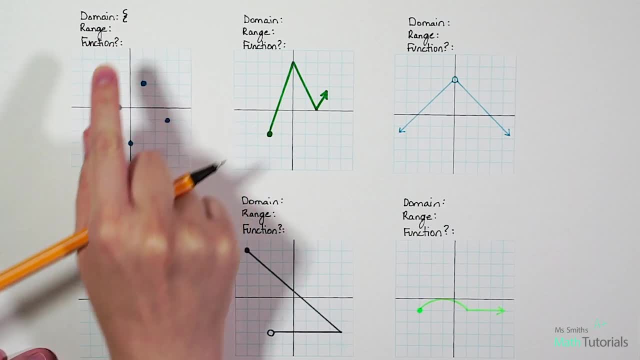 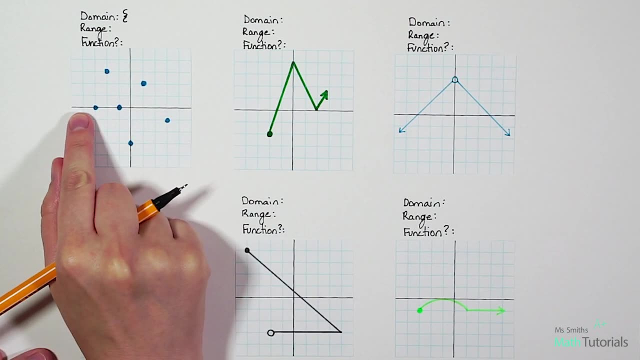 We do this little brace symbol And what we're gonna do is list out every x value, And I'm gonna do this value. So the easiest way to do this is to look at each point, kind of starting from the left and moving to the right, Look at each point and write its x value. 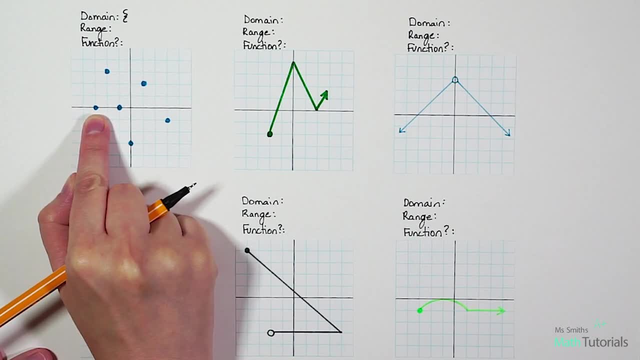 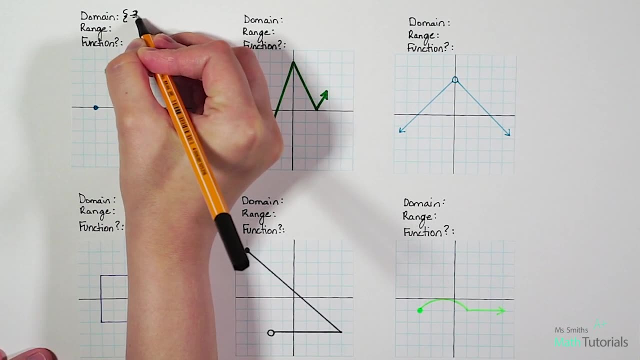 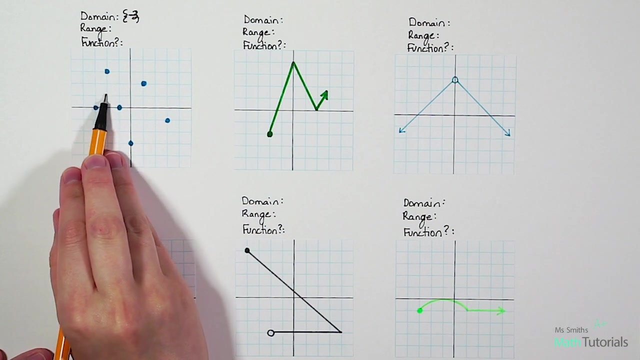 So for this first one, its x value is negative 3, right Negative 1, negative 2, negative 3.. It's a terrible 3.. And then the next point we cross would be this one, and that one falls at negative 2.. So we write negative 2.. 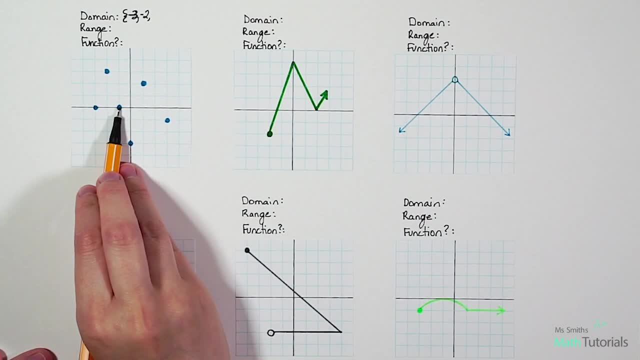 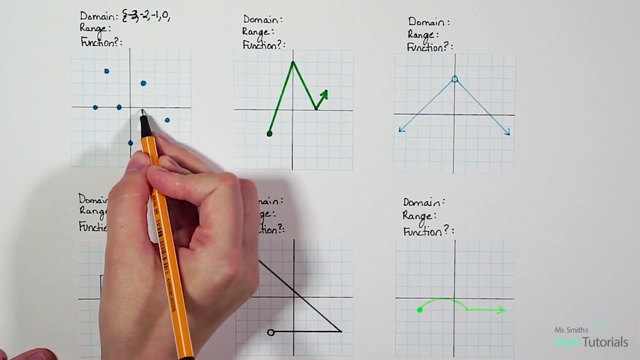 Our next point would be here, which falls at negative 1.. Remember, we're looking at the x-axis. Our next point would be here, which falls at 0 on the x-axis. Our next point would be here: that falls at positive 1.. And our 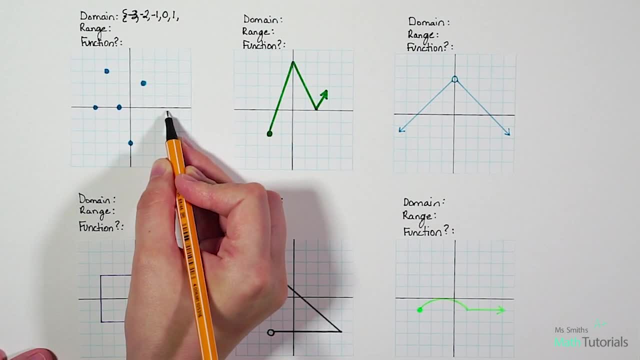 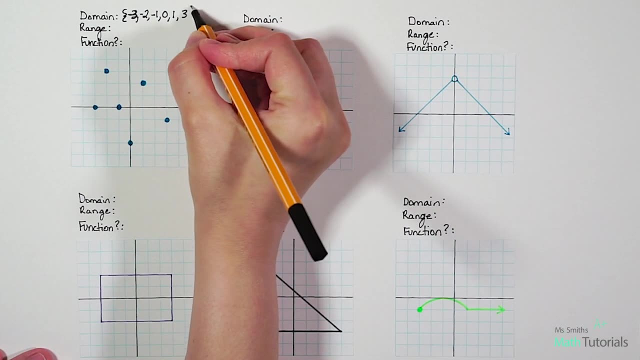 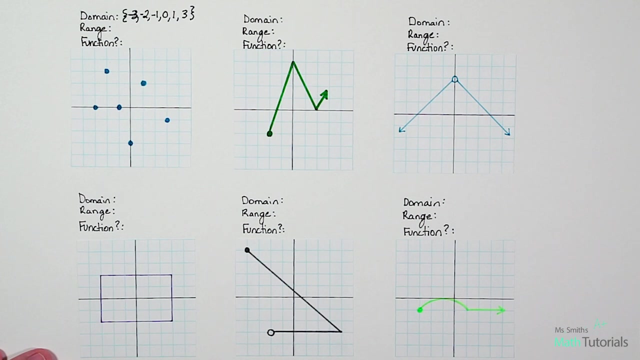 last point would be here, which falls at negative 1.. And now that we've listed out all the x values that we see, we close our brace And you're done with your domain. Now for the range, we're going to do the same. 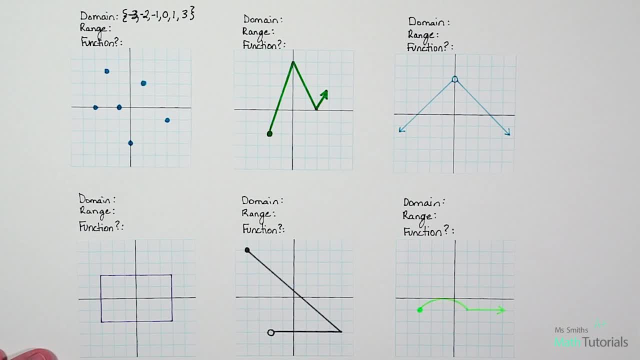 thing, but this time we're gonna list out all the y values of each point. So again, we just create our brace. It's showing that this is a set we're creating And let's start from the bottom and move up. So 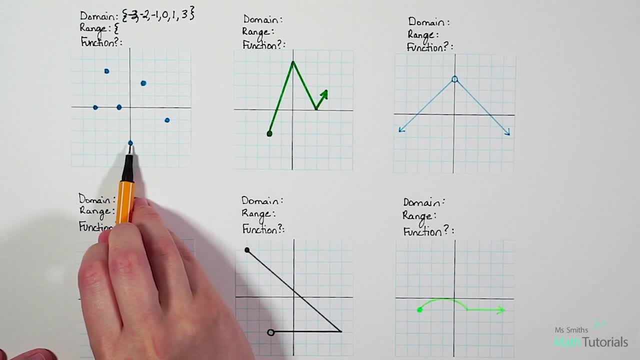 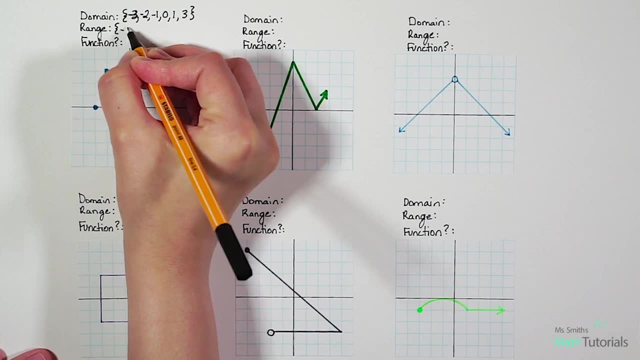 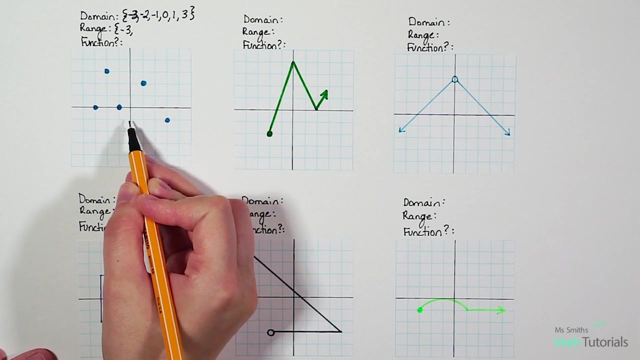 this lowest point. what is it on the y-axis? Because range means y, So on the y-axis it's falling at negative 3.. Our next point up would be this one: here, What is it on the y-axis? It falls at negative. 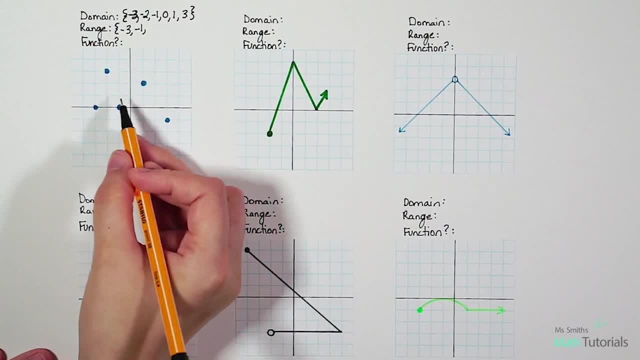 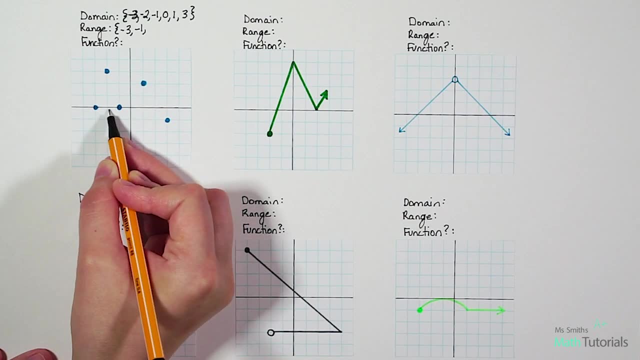 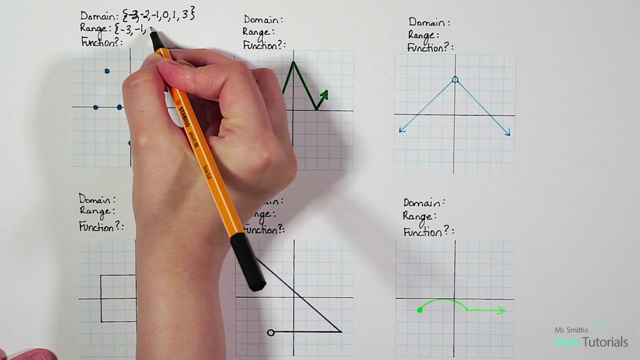 1.. Our next point would be: both of these, right, They're even along the y-axis and they both are falling at negative 3.. So we're going to do the same thing here, which falls at positive 0.. So we do not need to write 0 twice, we only need to write 0 one time. That covers both. 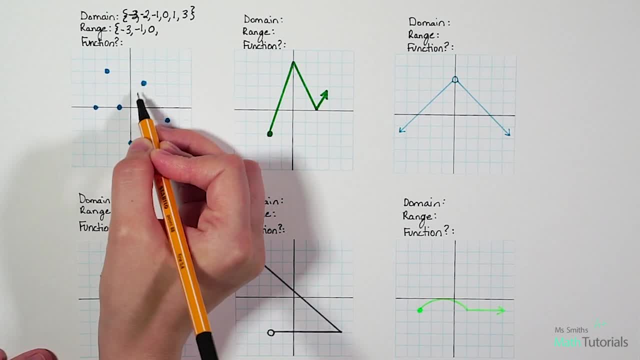 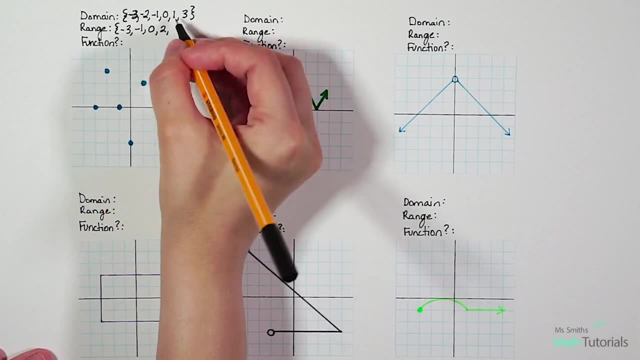 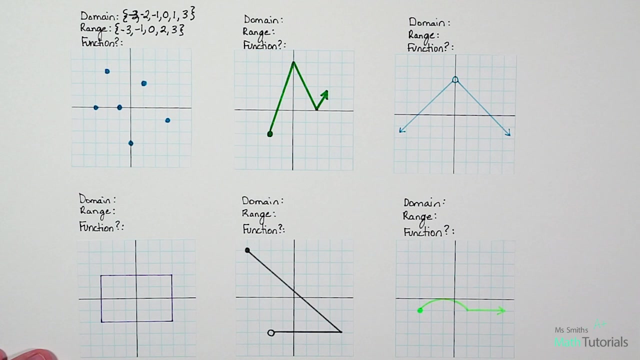 of those points. Now this one: our next point up would fall at positive 2, and our last point would fall at positive 3.. And then our range is done. Now, is it a function? So, when What we want to do is just kind of, at each point, just make sure, is each point only crossing my? 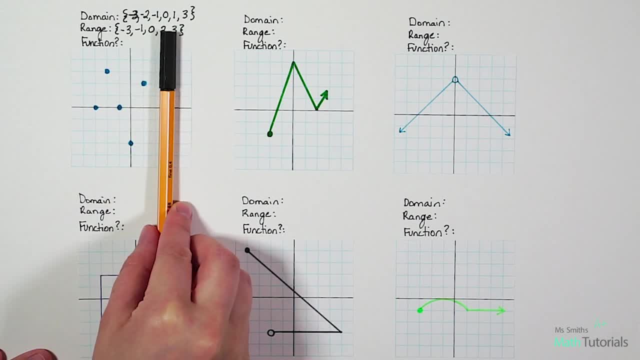 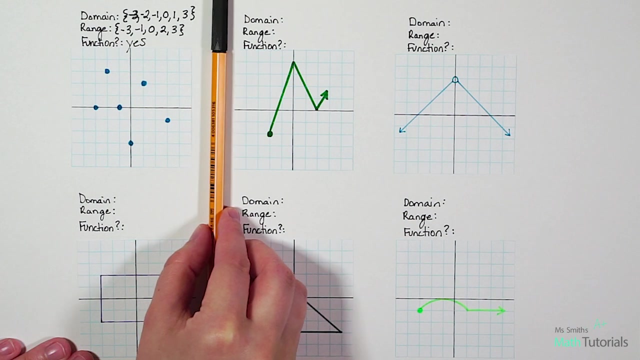 vertical line once right, We don't have any repeat x values and in this case we don't. So, yes, this is a function For this example. when we do our domain, we're going to go back to reading left to right. So when we come in from the left, what's the first place we hit? 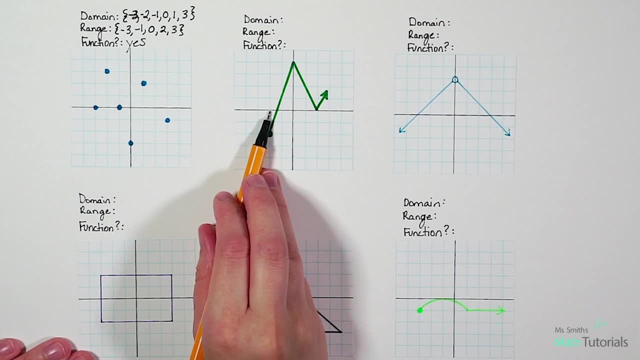 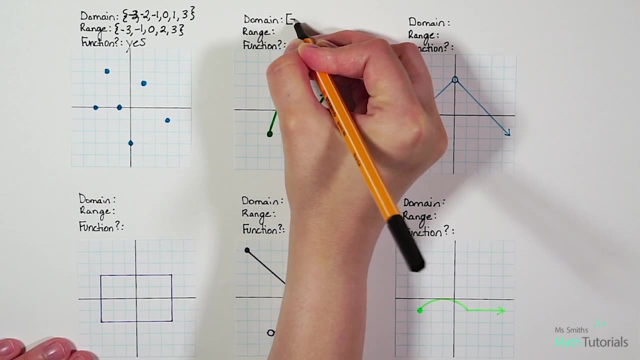 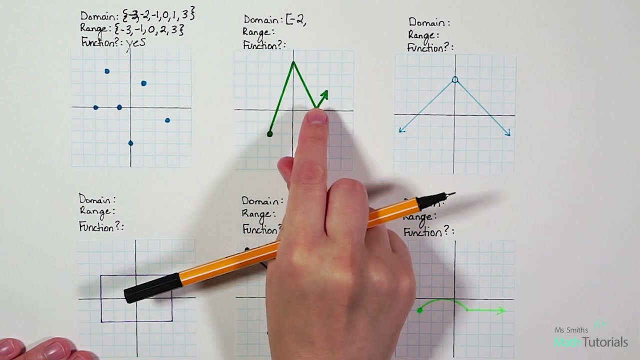 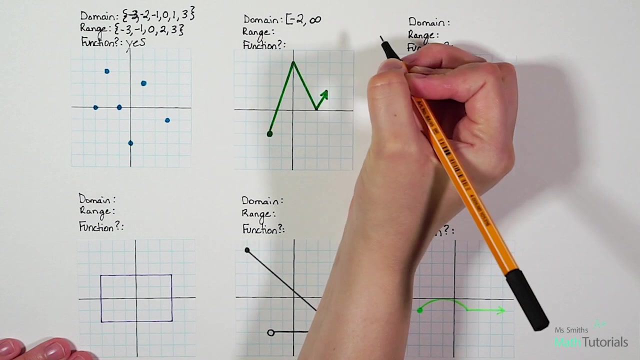 It's a solid point at negative 2.. Remember, we're looking at the x-axis for domain, So a solid point gets a bracket negative 2.. Now, when we come in from the right, what's the first place we hit? It's an arrow, and an arrow means infinity. It's on the right, so it is a positive infinity. 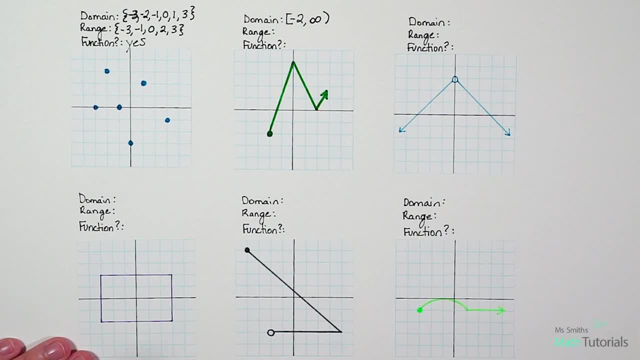 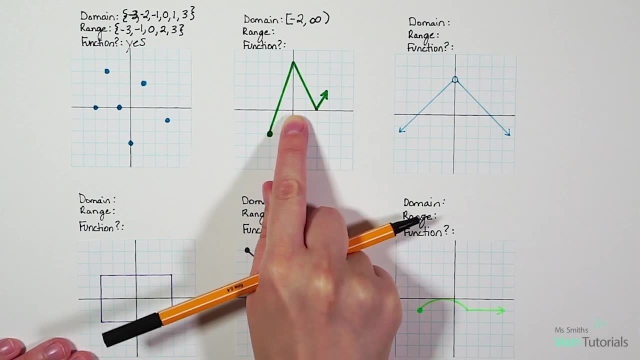 and infinities always get parentheses. Now for our range. Let's go back to reading left to right, From the bottom up. so the first place I hit is a solid point at negative 2.. So we get a bracket negative 2.. 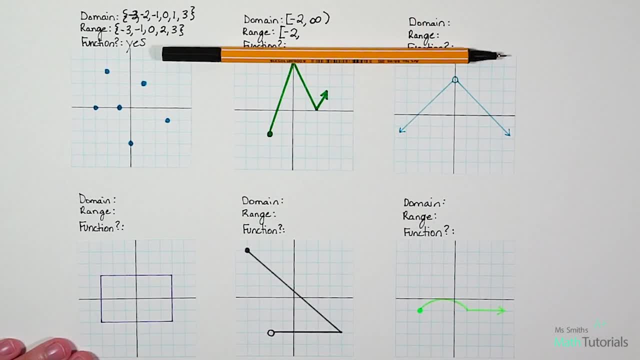 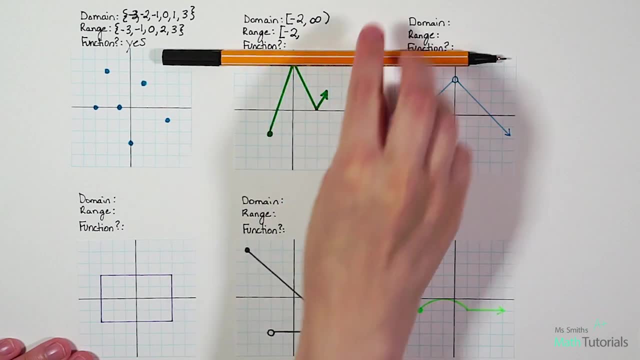 When we come in from the top. I've purposely made this one a little tricky because a lot of people may say, oh, the first place we hit is a positive 4. And if you just glance at it, they'd be right. that does look like the highest place on our. 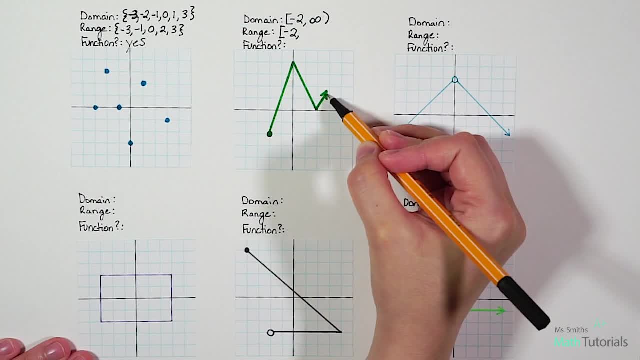 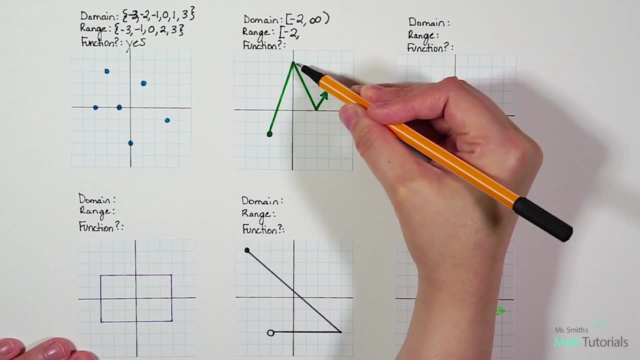 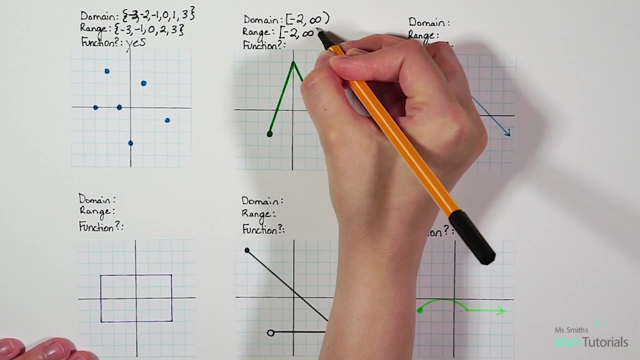 graph, But we see this arrow down here. Now that arrow is going to keep going up forever. It's not going to stop at positive 4. It's going to go up forever. So this one is actually positive infinity, with a parenthesis. 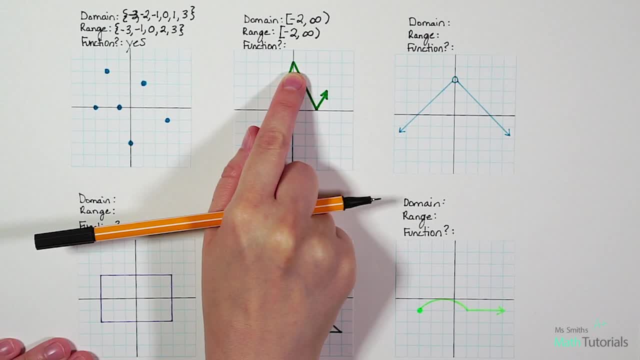 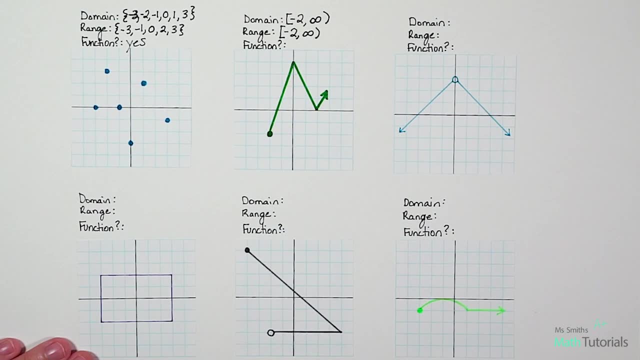 So sometimes they try to trick you and the first thing you touch isn't actually the answer. So you want to make sure you're looking at the picture as a whole. Now is this one a function? Does it pass the vertical line test? Yes, it does. 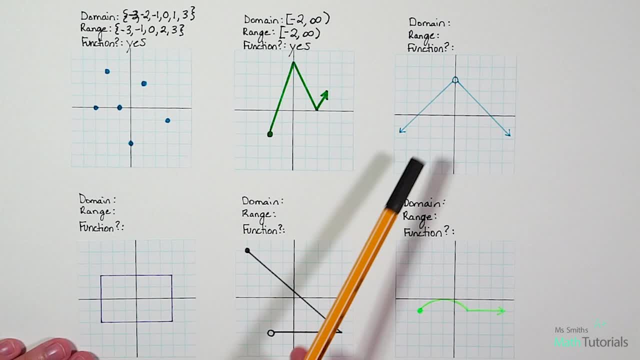 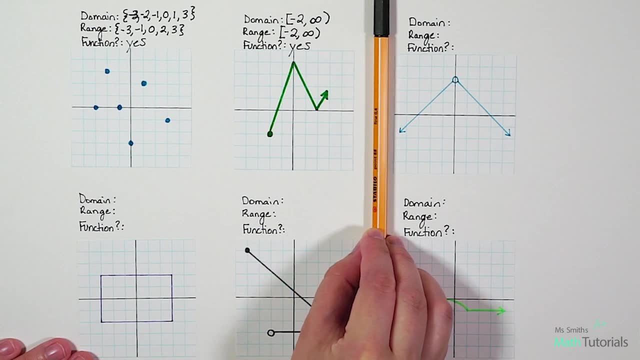 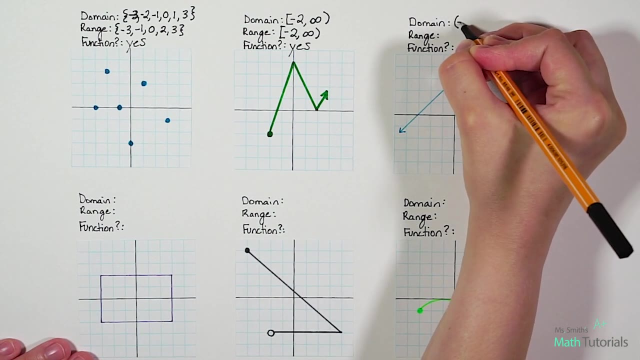 So, yep, it is a function. This next example is probably the hardest one on the sheet. When we do domain and we pull in from the left, the first place we hit is an arrow. So we can go ahead and do our parenthesis, negative infinity, because it's on the left. 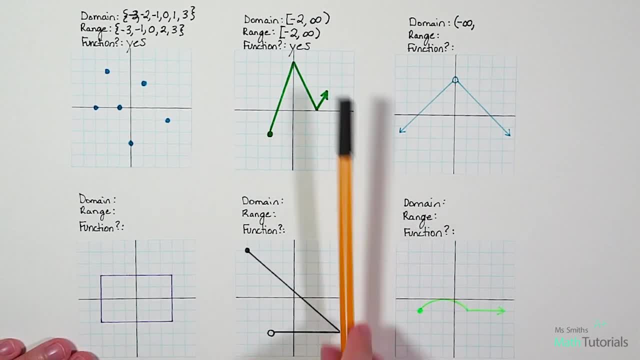 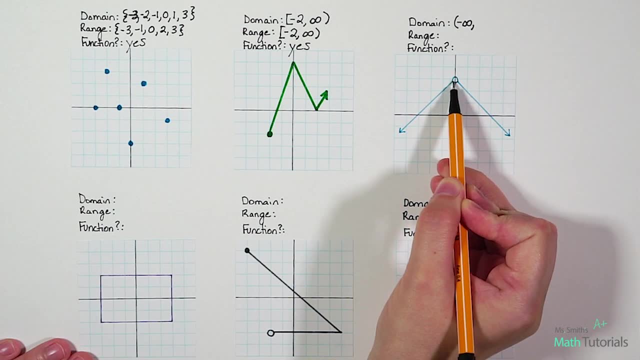 and our comma. Now, before we immediately do that, We need to immediately jump over and come in from the right. We need to notice something. We've got an open circle in this graph and it's happening where x is zero, x is zero right here, and that is a what we call a hole in the graph. 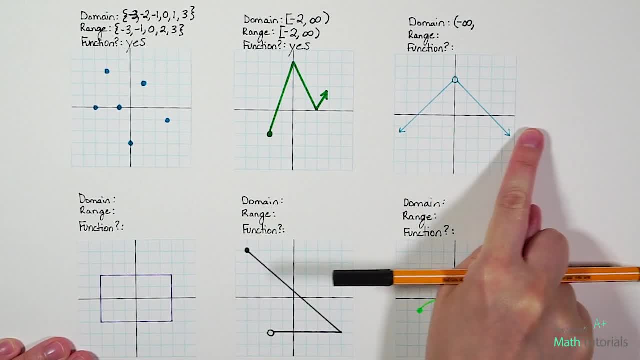 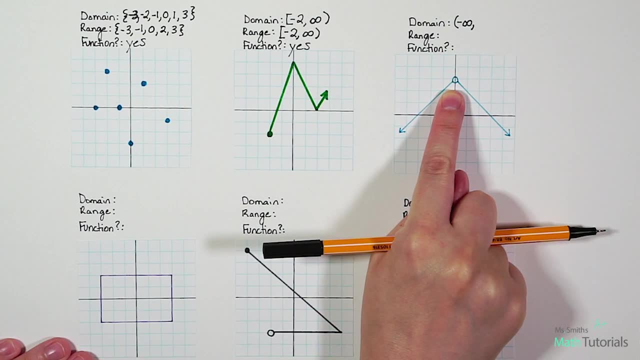 Okay, because it looks like it's going to be an all real numbers, but yet we have this hole here, And that hole is a non-included point. So there's a point here. There's a point here, A formal way that we could write this. 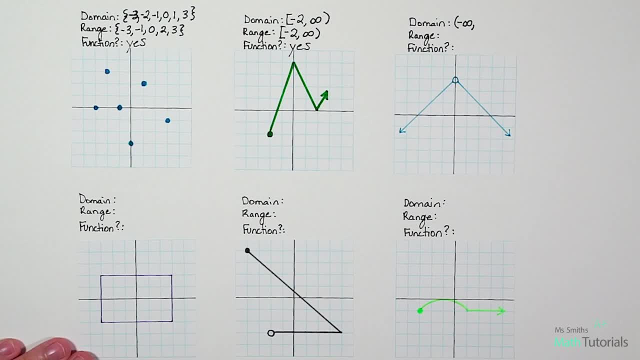 And then there's kind of like an easier informal way. So I'm going to start by showing you the formal way. We got our negative infinity on the left And then what's happening is: it's all real numbers until we hit this hole. 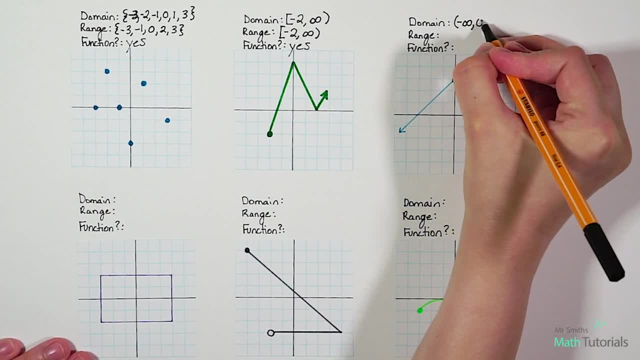 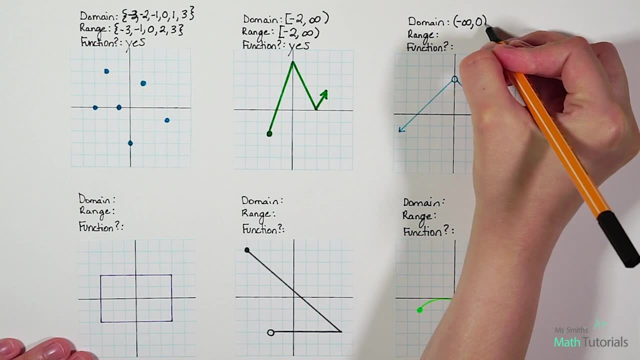 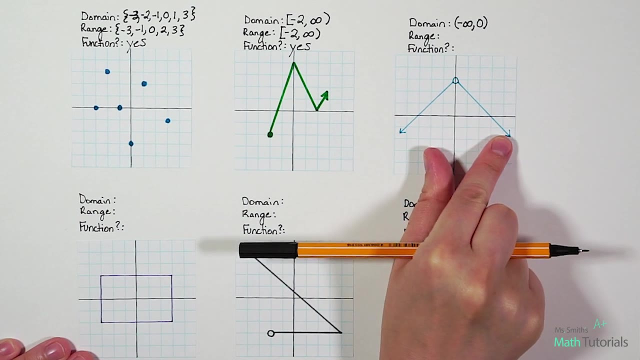 That hole is occurring at zero, So we're going to put zero. And it is a non-included point. It's an open circle, So we're going to close it with a perfect Parenthesis. Now the graph picks back up with a solid line and it continues on for infinity this way. 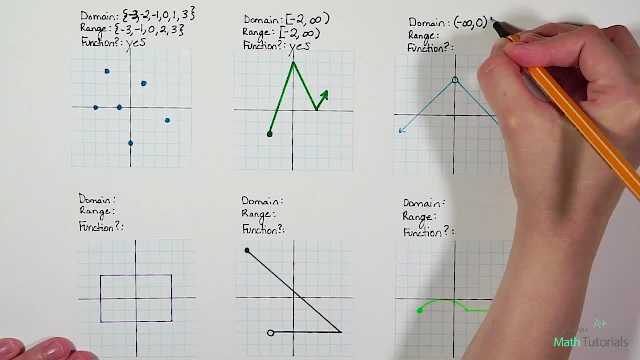 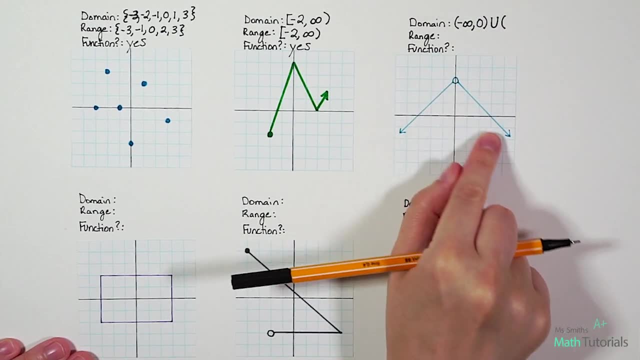 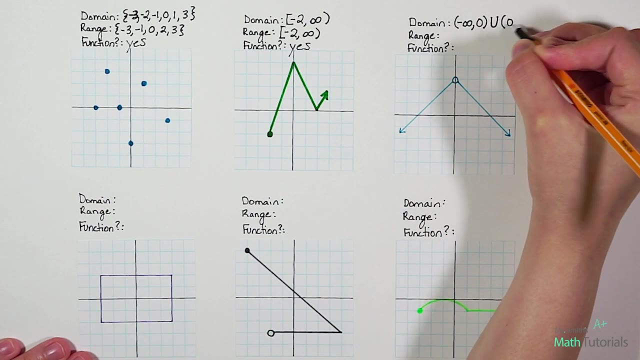 So we can show that the formal way is by putting a U, A capital U, which stands for a union, And then showing the second part. So the second part picks up at zero. It's a non-included point. So again it gets a parenthesis. 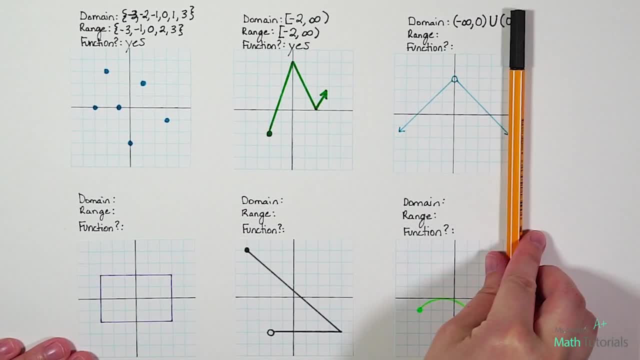 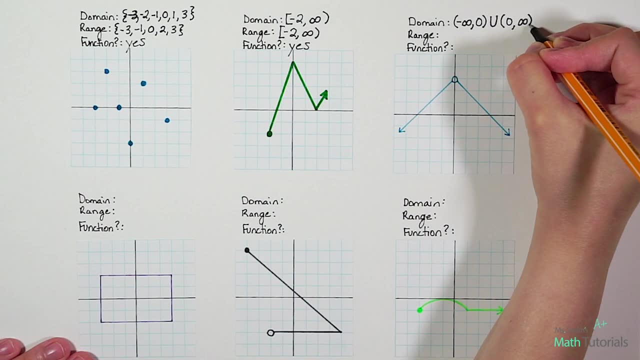 And it goes all the way To our right side, which is an arrow infinity, And it's on the right, so it's going to be positive And infinities always get parenthesis. That is the formal way to answer. Now the informal, kind of shorthand way would be to say: this graph goes from negative infinity. 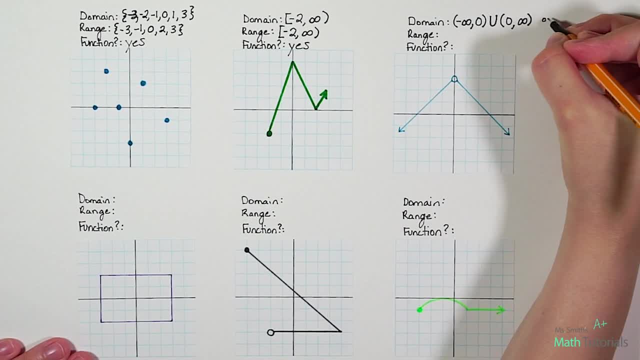 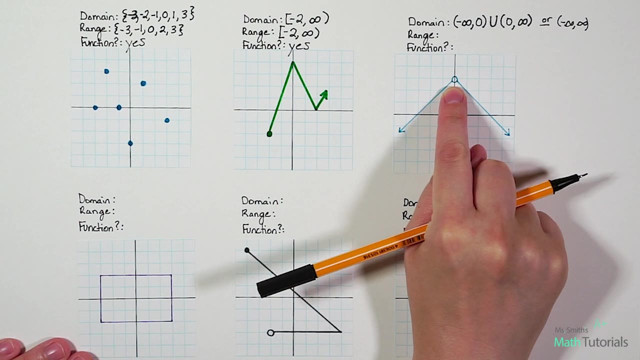 to positive infinity. So I'm going to do like a little, or because this is our other option. So we could go Negative infinity to positive infinity, But we just need to add this restriction here that x cannot equal zero, So we could just add either below it or beside it. 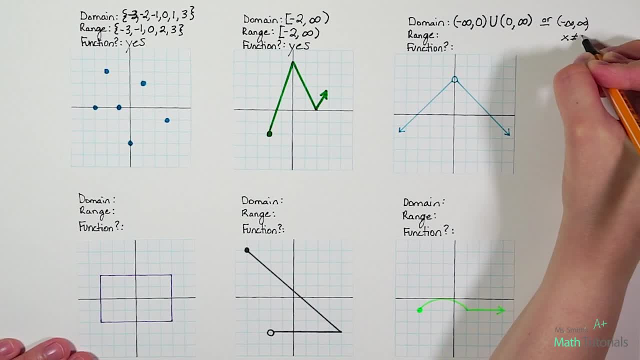 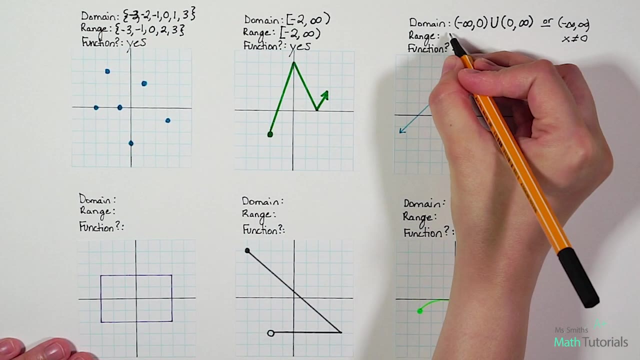 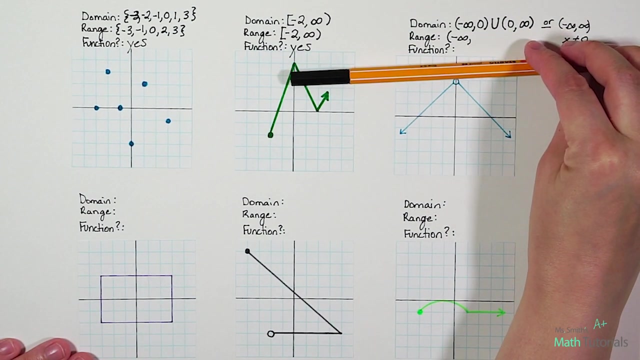 We could add: x cannot equal zero. So again, formal way, less formal way. So the range, remember. we read bottom First and we hit a double arrow right. so negative infinity, with a parenthesis. And when we read it from the top, coming down the first place, we hit. 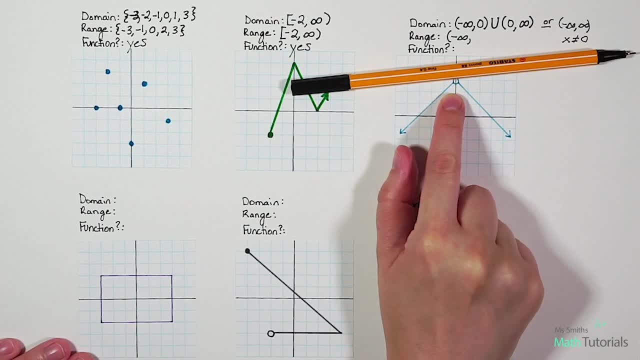 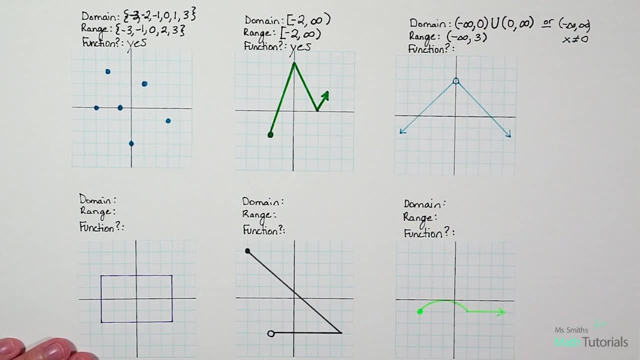 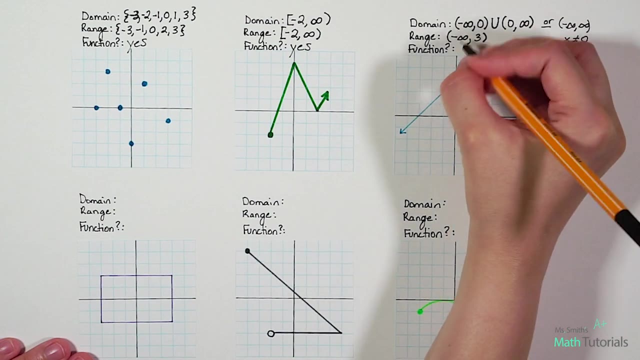 Is an open circle at positive three, So we can put positive three And it, because it's an open circle, it gets a parenthesis. Now is this a function? Well, does it pass the vertical line test? It sure does. So, yes, it is a function. 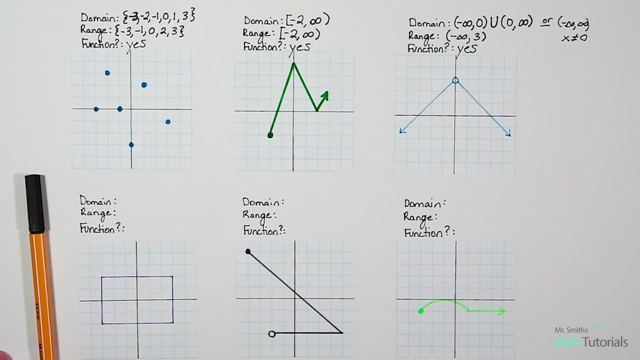 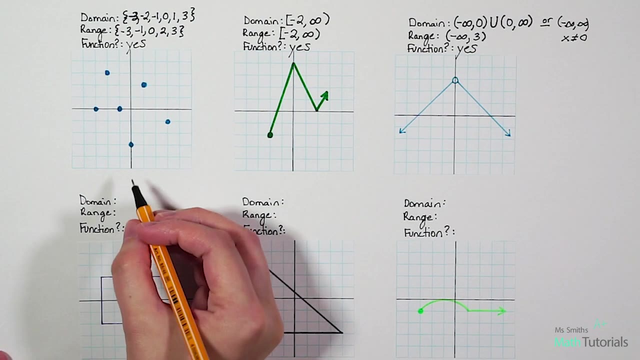 For this example, when we do the domain and we start from the left And pull in, the first place we hit is actually a solid line right, But it's a solid line at negative three on the x axis. So remember: solid lines get brackets. 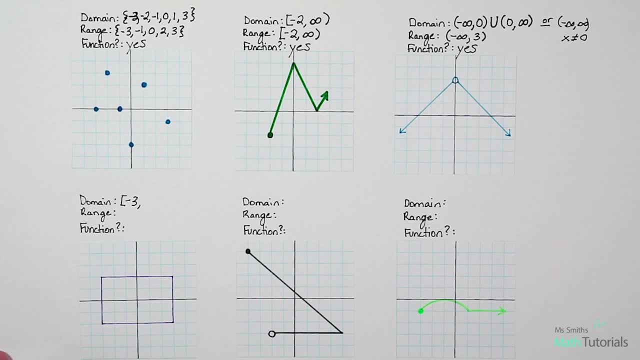 And it is at bracket negative three. And then, when we read this from the right, We hit another solid line at positive three And again solid lines get brackets. When we do the range, We see that the first thing we hit is a solid line at negative two. 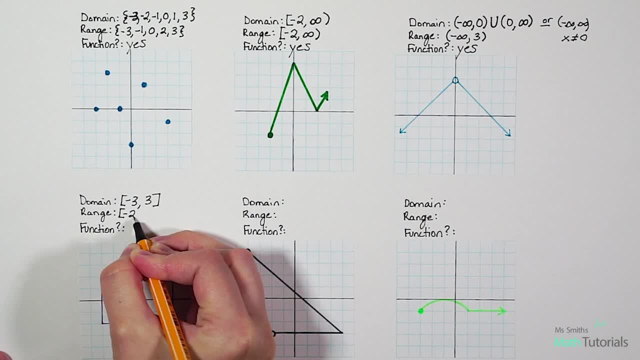 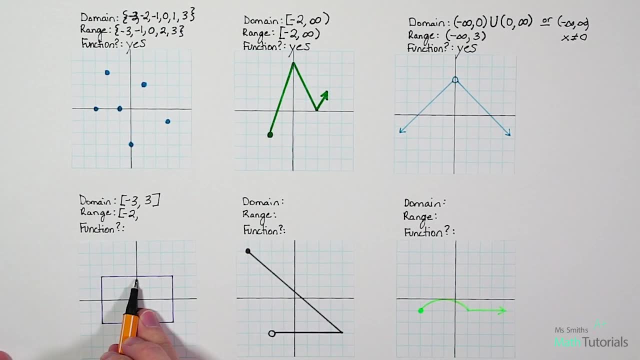 So we have a bracket, negative two, And then, from the top, We also hit a solid line at positive two. So solid lines get brackets. Now is this one a function? So far, all of our graphs have been functions, But for this one we finally get to see one where it's not a function. 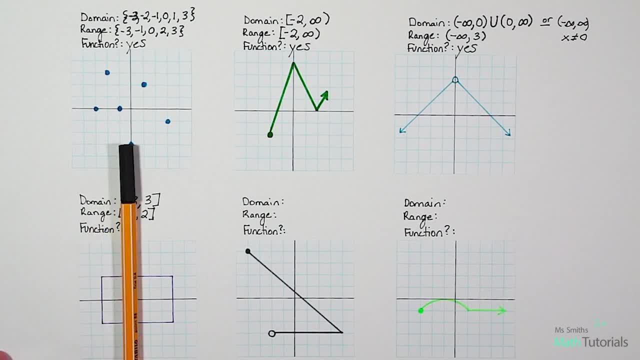 And let me show you why. When we run our vertical line through the graph, Do you see that it hits the purple line, hits the pen, more than once at a time. If that happens even once right here, it happens throughout the entire graph. But if it happens even once, 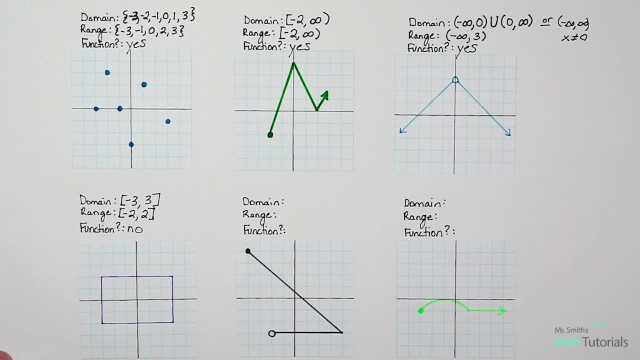 This is not a function. For our next example, When we come in from the left, We first hit a solid point And on the x axis that solid point falls at negative four. So we go bracket negative four. And then, when we come in from the right, 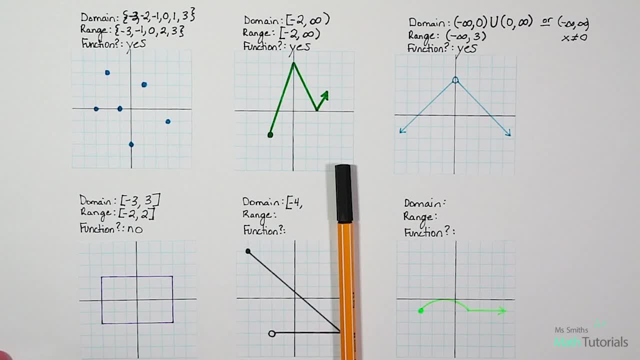 The first thing we hit is a solid. This is more like a solid line. We don't see like a definitive point, But it is a solid point there And it's a solid point at positive four. So it also gets a bracket. 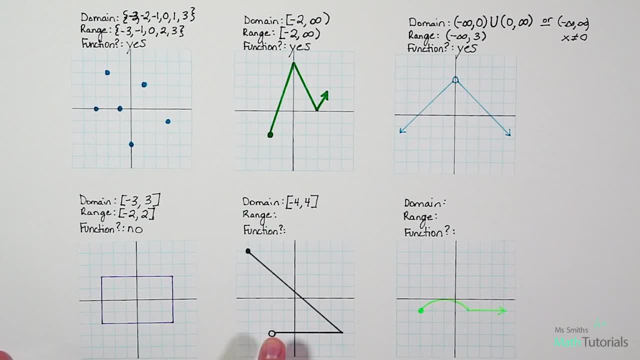 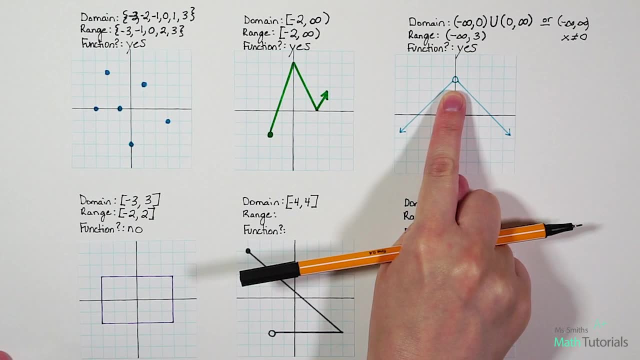 Now I know some people may be wondering. But wait, there's an open circle in there, Kind of similar to this one Where we talked about how there was a hole in the graph That we needed to address in our answer. Now, for this one, though, we actually don't. 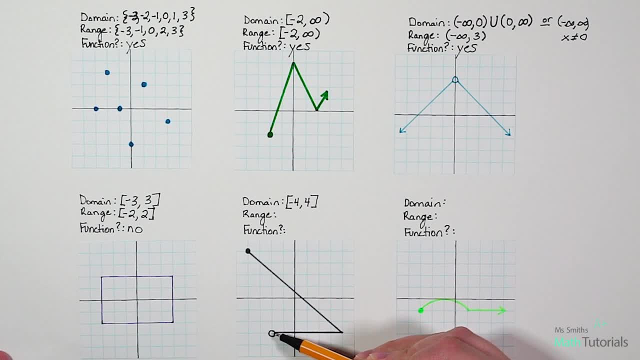 And the reason why is, Even though we have this open circle- And remember it's the x values we're looking at- This one has an open circle at negative two, But if we look This graph also extends up here at negative two. 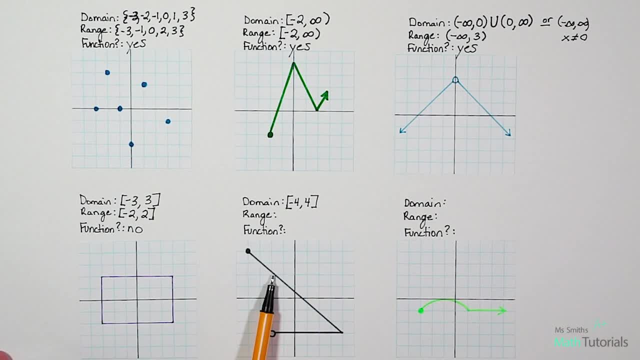 And it's a solid line. So that solid line actually covers that open circle. So even though it's open here, It's not a true hole in our x values Because It's covered by that solid line up here. See, we didn't have that here. 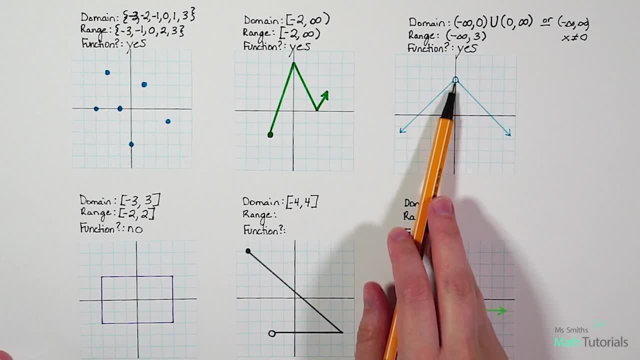 It was just an open circle And there was nowhere else on our x axis That covered it where x was zero. So a little bit of a different situation here. Now for our range. When we pull up from the bottom, The first thing we hit is a solid line. 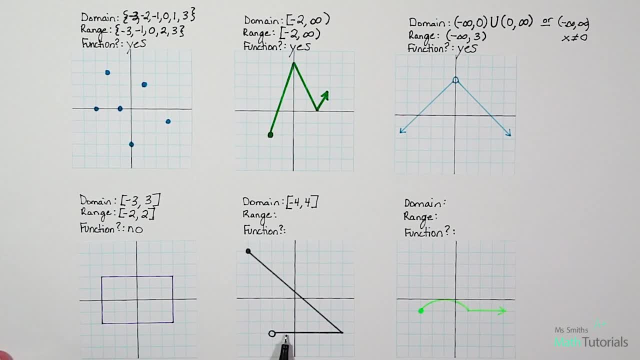 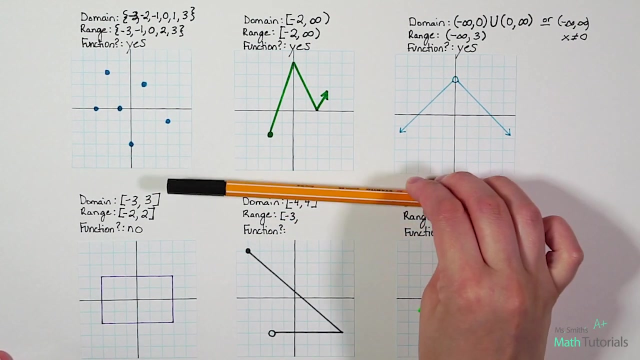 Now again, it's got this open circle here. But a solid line Wins over an open circle. This one would get a bracket. And where is it a bracket? Well, where is that solid line? It's at negative three Now, when we pull from the top. 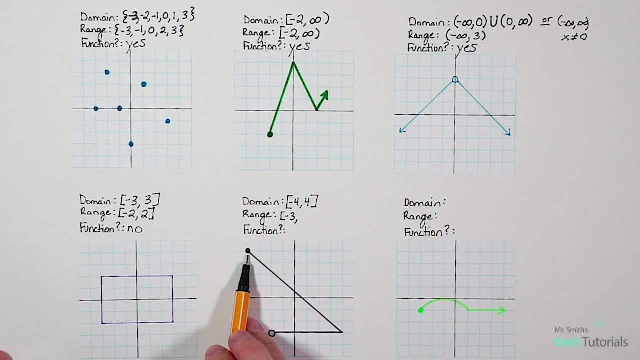 What's the first place? we hit A solid point at positive four. Is it a function? Well, does it pass the vertical line test? And right here we say nope, Right, all through here, It would hit my vertical line more than once. 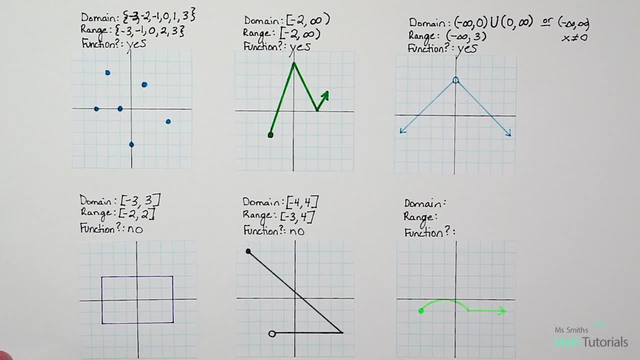 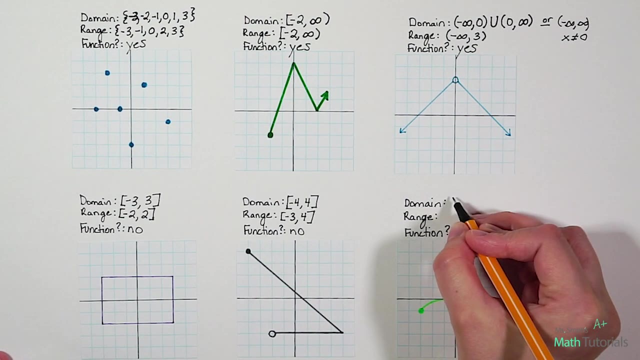 So this one is not a function. Okay, let's do one last example together For this one, our domain. When we pull from the left, What's the first place we hit? Well, it's a solid point where x is negative three. So we have a bracket: negative three. 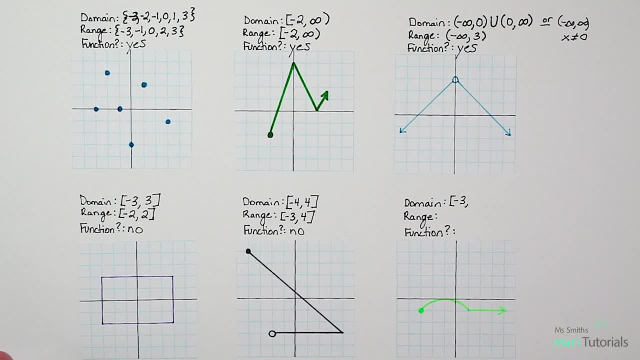 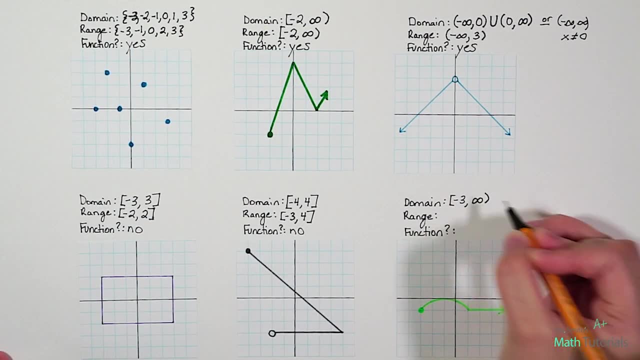 And then, when we look from the right, The first thing we hit is an arrow, And an arrow means infinity. It's on the right, so it's positive, And infinities always get a parenthesis. For our range, This one could be kind of tricky. 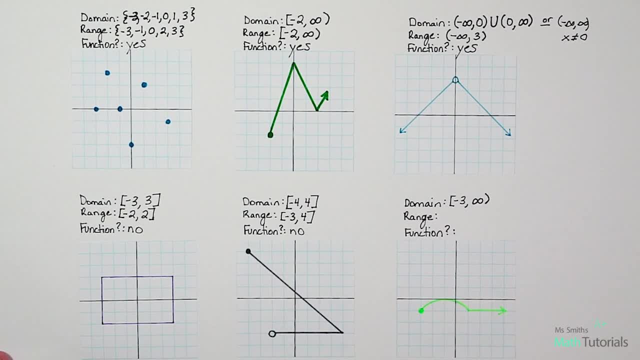 When we pull up from the bottom, The first thing we hit- Now we hit a lot here, Right, we hit a solid point here, We hit a solid line here, Which those are equivalent, So no big deal. But then a lot of people may get confused. 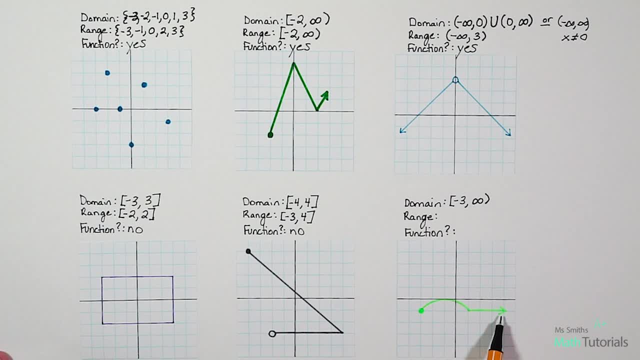 Because they see we also hit an arrow. Now, this arrow is a little different, though. This is not an arrow pointing down. Remember, for range, we're looking at the y-axis. This arrow is pointing to the right And it's going straight out to the right.